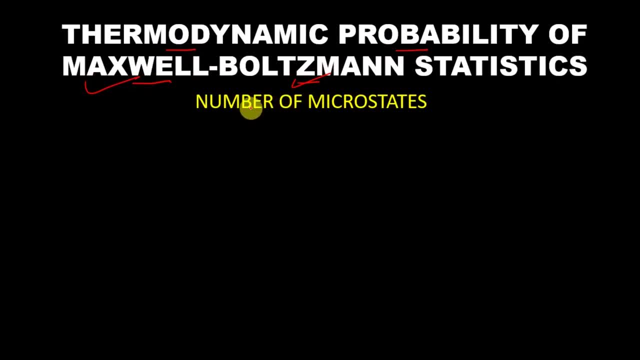 and so on for the other two. So let's get started Now. similar to the previous video, we will imagine boxes which are nothing but energy, like this. So let's get started Now. similar to the previous video, we will imagine boxes which are nothing but energy, like this: 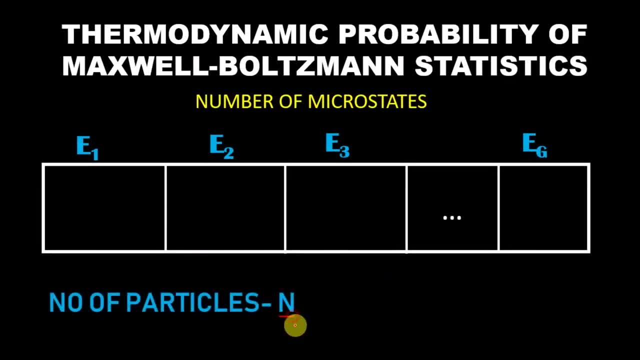 So let's get started And let us say we have the number of particles, which is n. Now what these functions basically tell us. See this, Let us say this is energy and this is the number of particles. okay, So like, the Maxwell-Boltzmann distribution function is something like this: 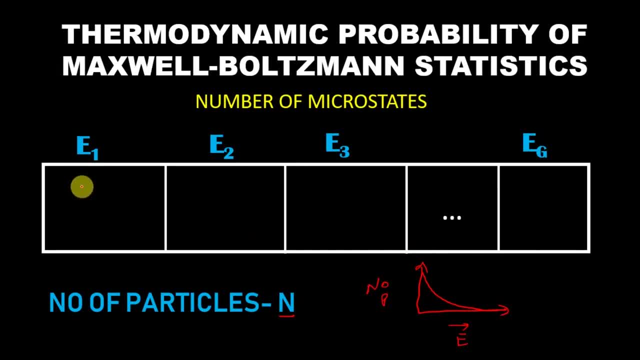 So what? these are basically telling us that how many particles are there in this one? how many are there in this one? how many are there in this one? These boxes are basically the energy levels. This axis is that energy and this distribution is the Maxwell-Boltzmann. 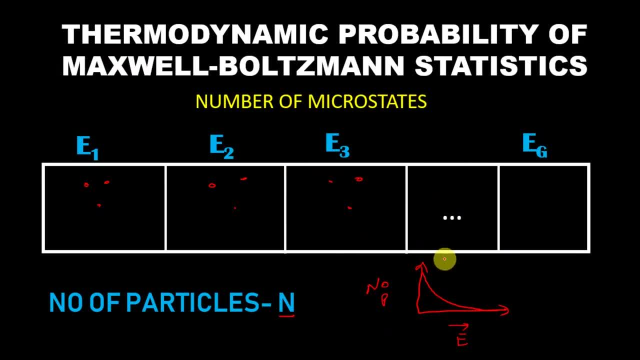 distribution function. So we need to derive this Now. to derive this, we will first assume that this box contains n1 particles, this box contains n2,, this box contains n3, and so on, to this box contains ng particles, And then we will apply. 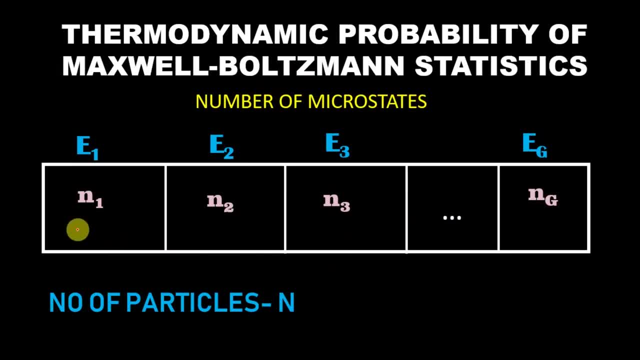 the conditions for a Maxwell-Boltzmann distribution function and we will see how this n1, n2, n3 will look like Like. first we need to find the number of microstates, that means the number of ways in which these n particles can arrange in here, and then by maximizing it we will get the most. 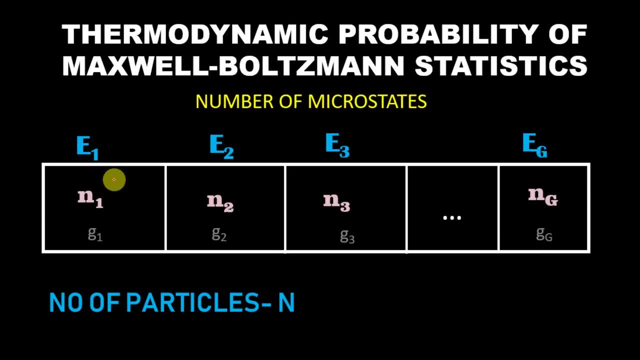 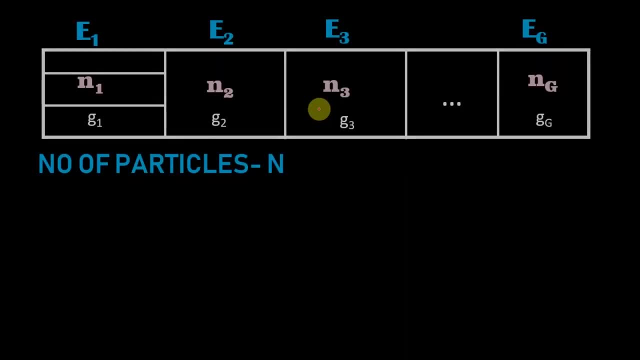 probable distribution And also these energy levels can be degenerate. that means there is a splitting of energy levels. You can imagine this by further dividing this box in sub levels. So this is the main energy level and these are the degenerate energy levels. So what is the condition? 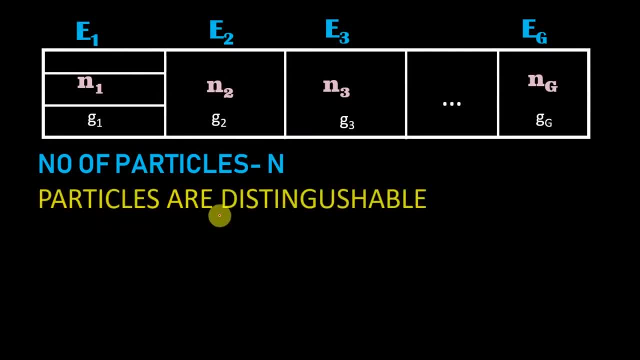 that the particles are. If we consider the Maxwell-Boltzmann statistics, that the particles are distinguishable, This is a really important thing. So let us take n distinguishable particles, like in here. we have taken 9 distinguishable particles. Now we need to find the number of. 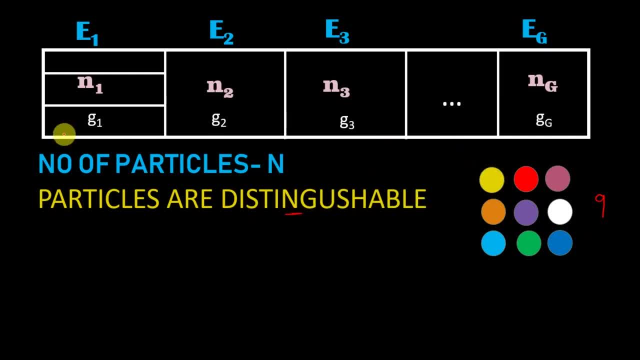 microstates. that means how these 9 particles can arrange themselves in these boxes. Now, first let us ignore this degeneracy, And ignoring this degeneracy will tell you later. so let us take an example. like we can choose three particles in here. 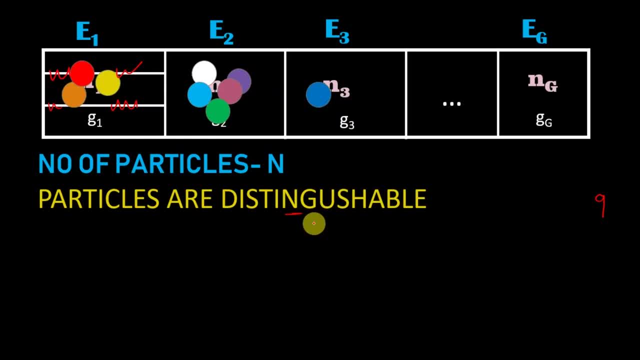 five particles in here and like one particle in here. now, if we ignore this degeneracy, that means that the further arrangement of these three particles in here won't count, because changing these won't change the microstate, won't change the arrangement, if we ignore this degeneracy for now. 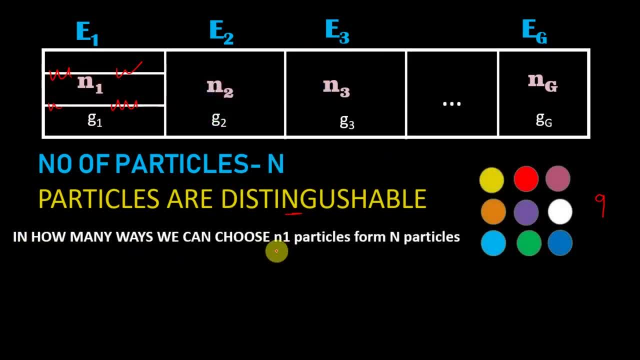 so the question in here is that: in how many ways we can choose n1 particles from n particles. now what do this means like? in how many ways we can choose n1 particles from these and particles like at first we will see it for this energy level. so in here, in how many ways we can choose this. 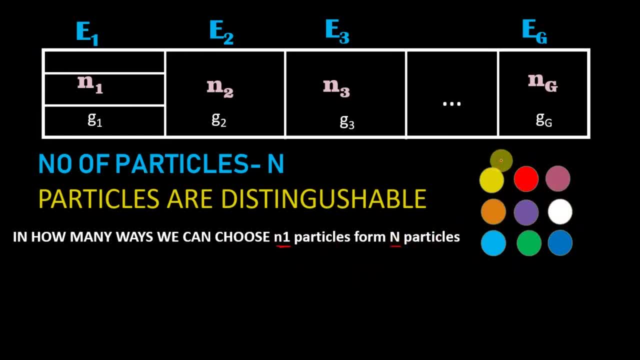 n1 particles from these n particles. like we can choose these three, we can choose these three and so on, but we have to remember that the further arrangement- like if we choose these three but these three will arrange them, so like if we choose this one at first and this one. 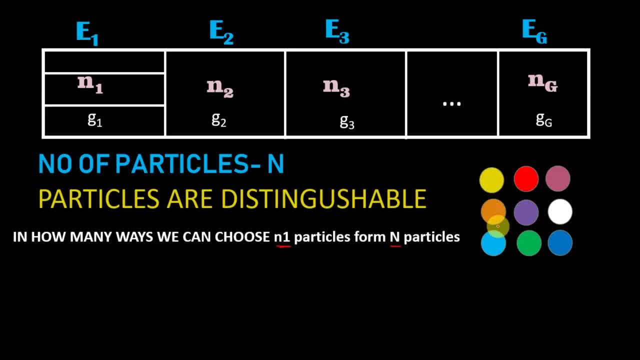 second one and this one third one, or this one first one, this one second one and this one third one. it won't change the microstate. so what is this? these are n particles and we need to choose n1 particles, so this is basically a combination. remember: note of automation. yes, the 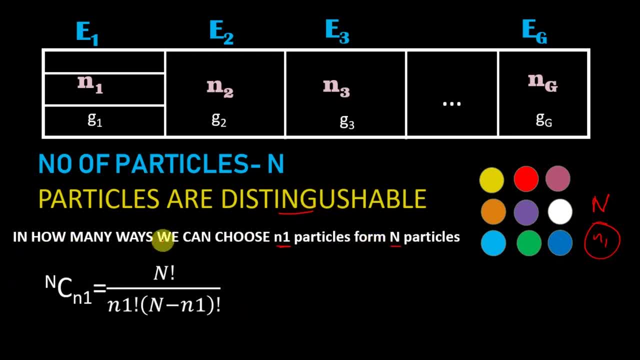 particles are distinguishable, but the one we are choosing are acting like indistinguishable particle, because in here the further arrangement won't count. yes, it will count when we will incorporate this degeneracy. okay, so this is a combination, like there are n particles and we need to choose n1 particles, so it 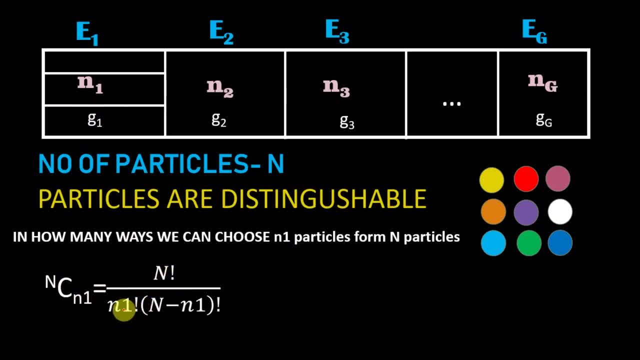 is nc n1, which is nothing but n factorial divided by n1 factorial, n minus n1 factorial. so this is for this energy level, the number of ways for this energy level. now this one is filled. now we have this energy level. now, remember, we have chosen n1 particles. so what we have left is this: n minus n1. 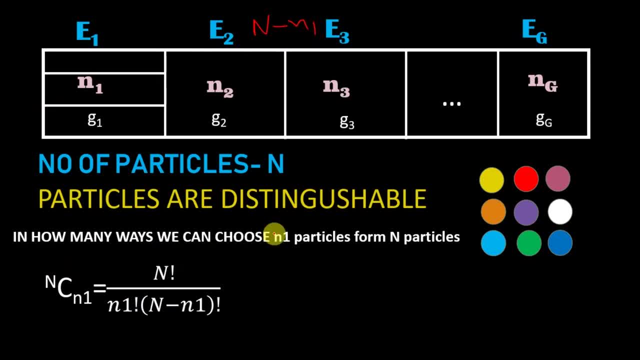 particles. now the question is in how many ways we can choose n2 particles from n minus n1 particles, which is this: that n minus n1, c, n2, that is, these are the number of particles, like in here, and this is the number of particles that we need to choose. so this is n factorial in here, that is. 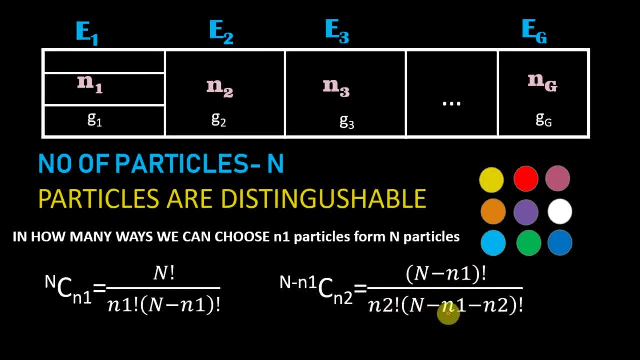 nue donation, one divided by n2 factorial, n minus n1 minus n2 factorial. now this is for this other N level and we will do it so on to eat Log. and now, if we multiply all those that the number of ways worry- 1, e2, e3- then what we will get is this: in How many ways these N? 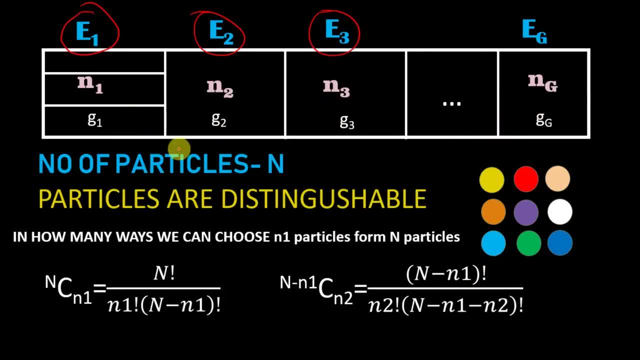 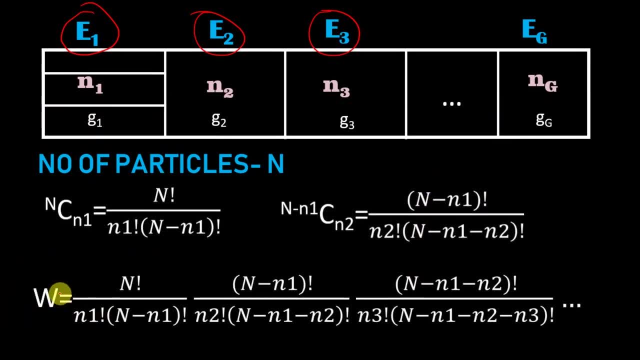 particles can arrange themselves in these energy levels. ignoring D generally worked in it W Now, which is equal to this multiply, this multiply by 4, e3.. Now in here, the number of particles left is n minus n1 minus n2, and so on. Now in here you can see. 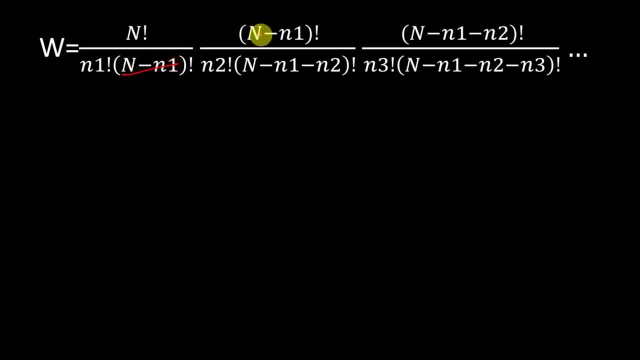 like this cancels this one, and this one cancels this one, and so on, And what we are left is this: which is n factorial divided by n1 factorial, n2 factorial, n3 factorial, and so on, to ni factorial and so on. Now we can represent it like this: that is n factorial divided by. this symbol is for: 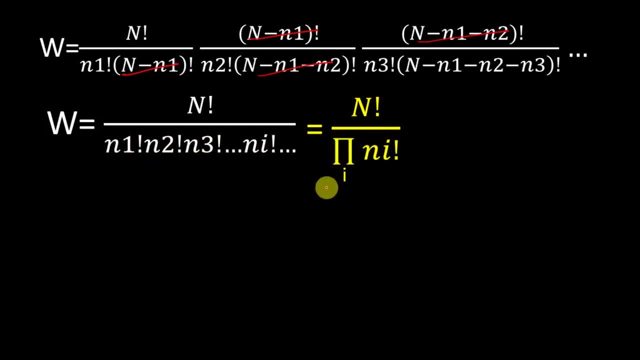 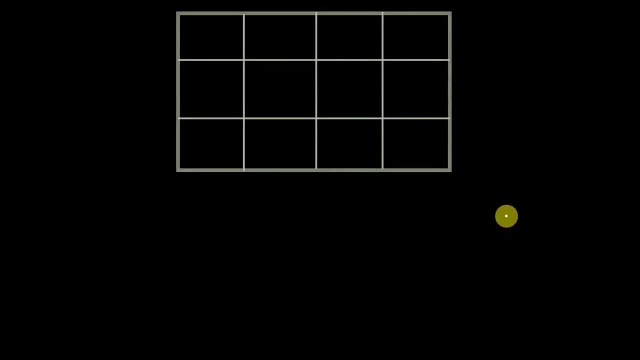 multiplication. So multiplication with the variable i and i, factorial. Now this is really important. This is one part of the answer. Okay, now we have to count the degeneracies also. Now to count the degenerate states, let us say: this is the energy box E1 and its degeneracy is: 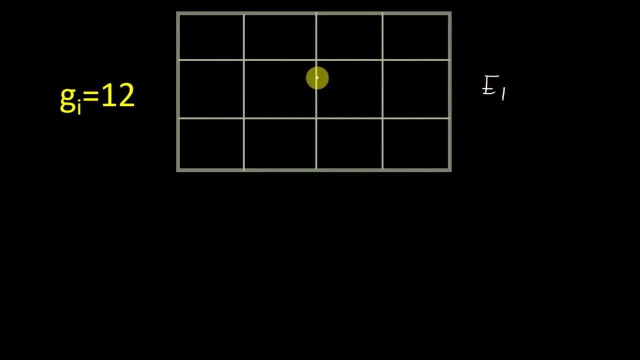 12. In here there are 12 sub boxes. Now the second condition of Maxwell-Boltzmann statistics is that there is no restriction on the number of particles in one box. That means in here there could be an infinite number of particles. So let us ask this question that if we have a one particle in here, 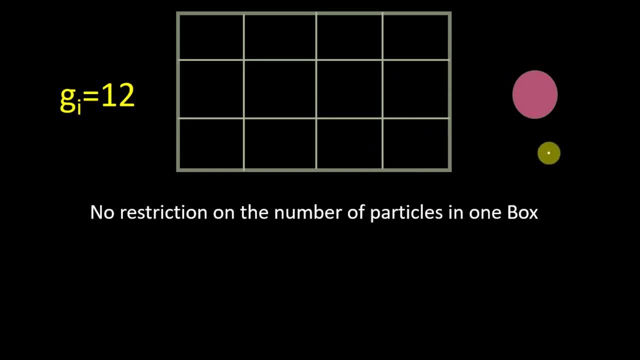 in how many ways it can arrange itself in here. And the answer is 12 ways, because in here this particle can either go in here, here, here, here, Okay, so the number of ways in which one particle can arrange in here is GI. Now imagine if we add 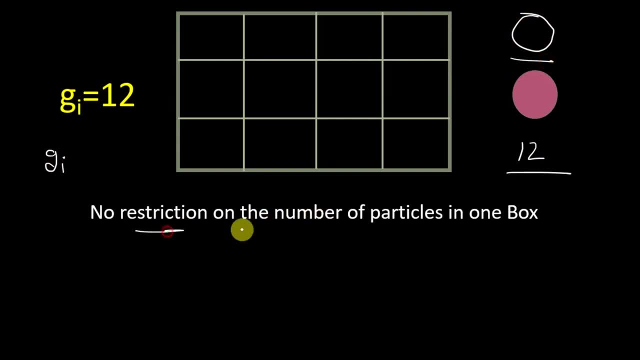 two particles, The second one, if there is no restriction, can also arrange itself in 12 ways. That means another GI. Now, if there are two particles, then they both can arrange themselves in GI multiplied by GI ways. That means GI raised to the power two ways If there are two particles. 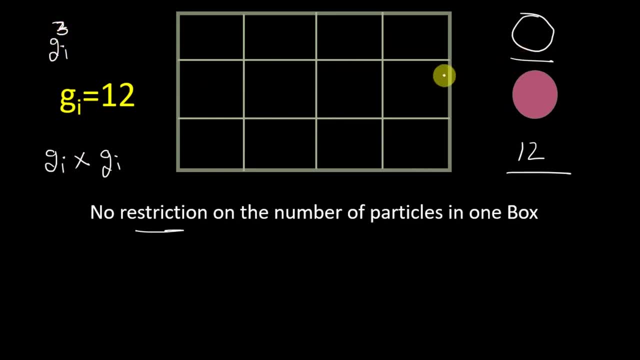 that means GI raised to the power three. If there are N1 particles then it means that GI raised to the power N1 ways. So in the first energy box, E1, the degenerate ways are GI raised to the power N1 and so on to energy box E2, E3 and so on, And if we multiply all those we will get the degenerate. 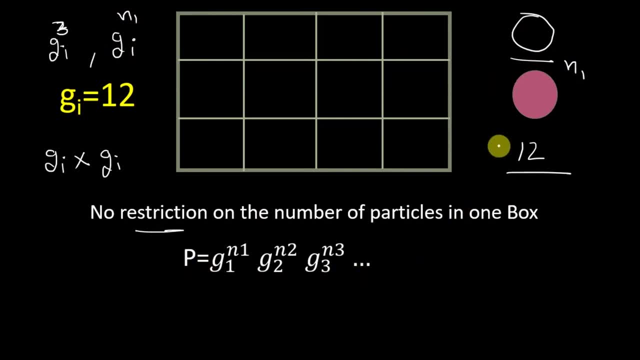 ways Like this is the ways with which those particles can arrange themselves in the degenerate energy levels. This is for the first box, E1.. This is for second box, E2, and so on. Now we can write it like this in here, like this: like this is the multiplication sign GI raised to. 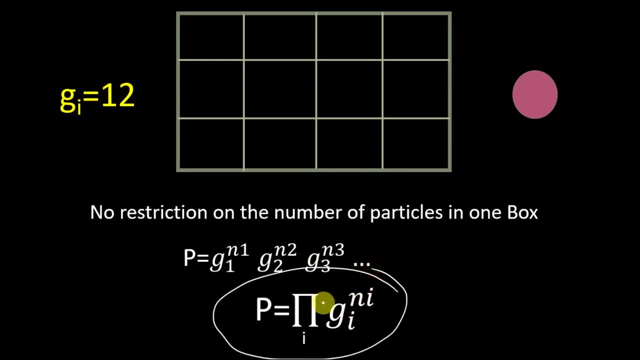 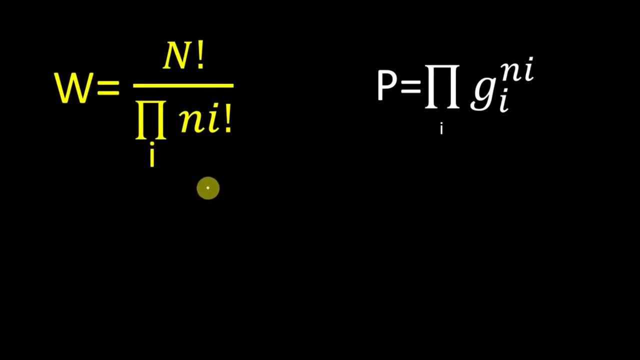 the power NI. Now, this is the second piece that we need Now. this is our first piece and this is our second piece. This is the number of ways those particles can arrange themselves in those energy boxes And this is the number of ways in which those particles can arrange themselves in the 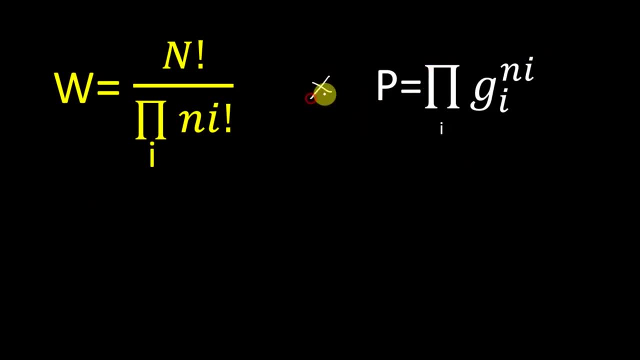 degenerate energy levels, And by multiplying these two we will get our answer, that is, the thermodynamic probability of Maxwell Boltzmann statistics. This is what we needed to find, And by maximizing this we will get our Maxwell Boltzmann distribution function. So this is our 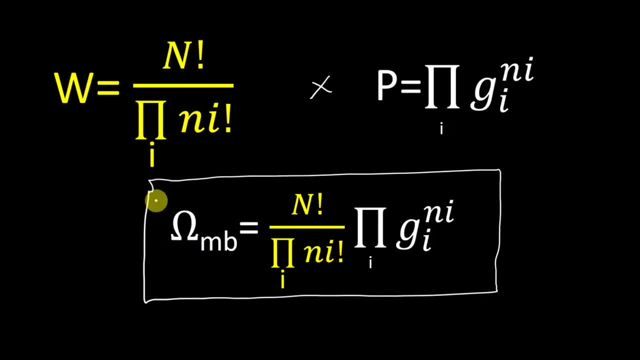 answer. Now also one thing: if you have watched the permutation and combination video In which we have like, converted from permutation to combination just by dividing by n- factorial, So in here, if you want to treat those particles as indistinguishable. Yes, we know that in classical 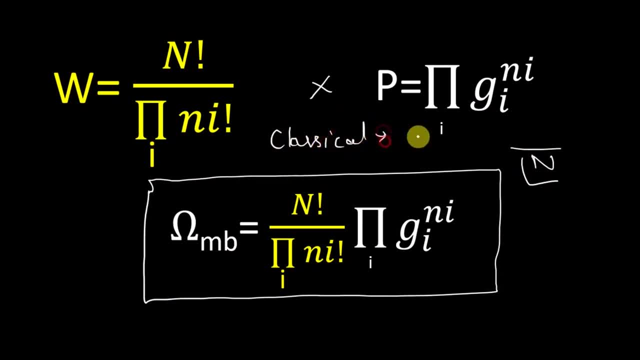 statistics, in classical statistics, the particles are distinguishable. Okay, Right, But sometimes, if you want to study like ideal gas, Then there, if we treat those particles as distinguishable, Then there is some paradox which arises that is known as Gibbs paradox. Okay, The paradox is that 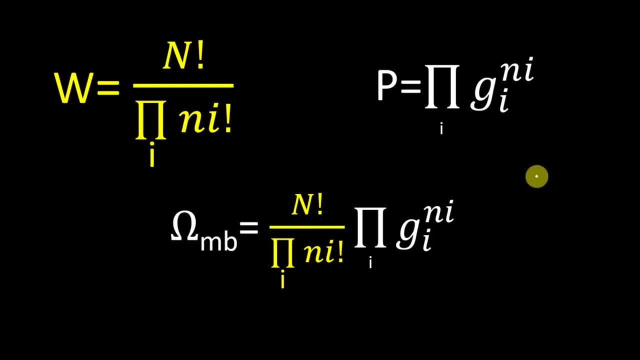 the self-mixing of gas. That means, when the gas is mixing on itself increases the entropy, which is we don't want There. we also use the Maxwell Boltzmann statistics, but with one change: dividing this thing by n- factorial. So this cancels this one. So this is four. 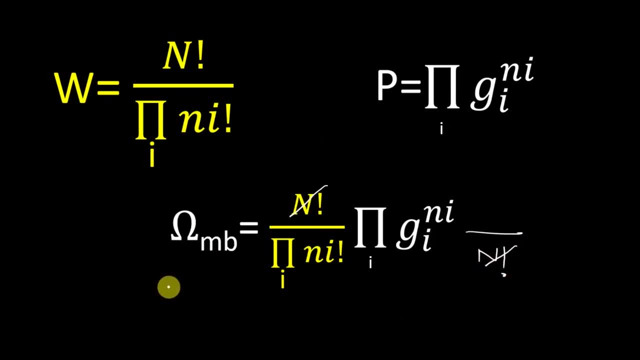 indistinguishable particles of Maxwell Boltzmann statistics. We want to treat it like this, But to derive the Maxwell Boltzmann distribution function, we will use this one. So this is our answer. Now, if you are in a hurry, you can just stop. 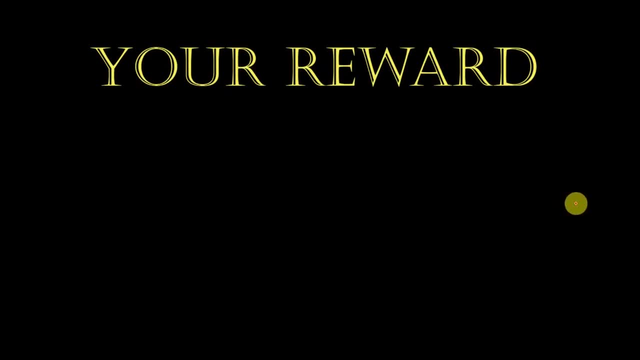 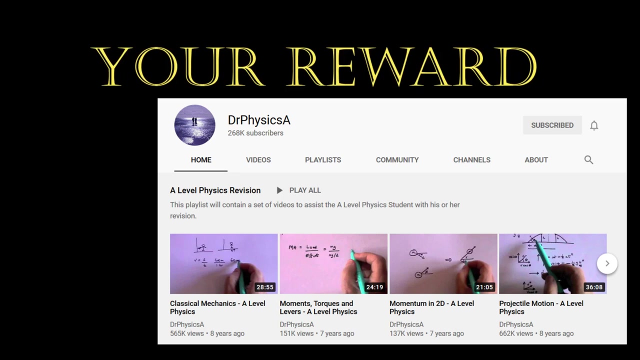 watching this video. This further video is not related to studies, And this is the first time I am ever doing this on this channel. Now, while studying electromagnetism on YouTube, I stumbled upon a channel named Dr Physics A And he taught electromagnetism really well. 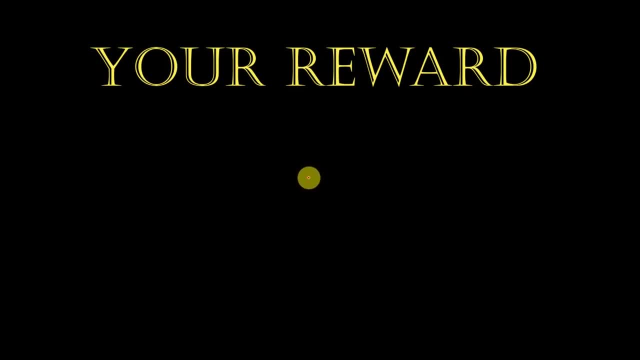 But I found a really unique thing in his work. He said that if you want to treat the Maxwell Boltzmann statistics- which I never saw another YouTuber do it- The thing is that at the end of his video, At the end of his video, he showed us cool things of his house, like his clock, his 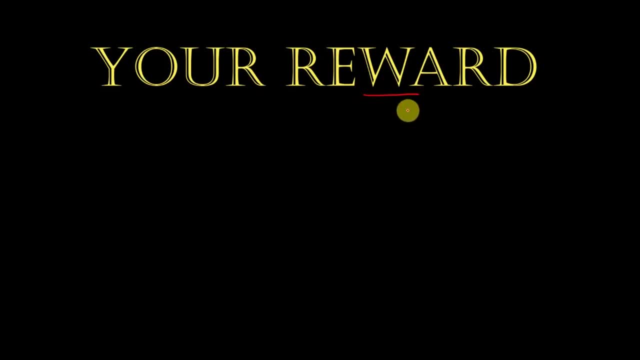 cats, etc. etc. A kind of reward for watching his educational videos. So I also thought that I can give you a reward on watching these educational videos on YouTube, Because the YouTube is filled with entertainment and other stuff, But you are studying. That is a good. 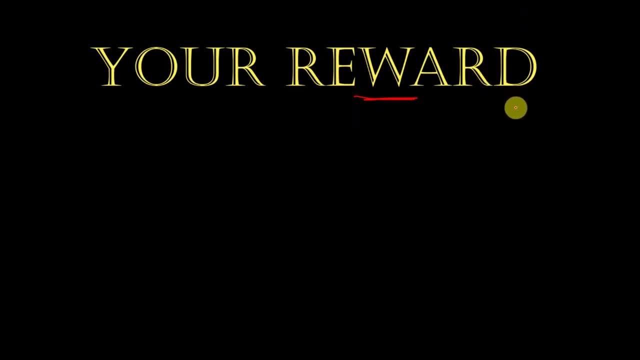 thing And you deserve a reward. So I say I hope you enjoyed this video And please Like, Share, Comment and Subscribe to my channel. Thank you very much reward. so if i also show you cool things of my house, it would be a copy, so i thought i can show. 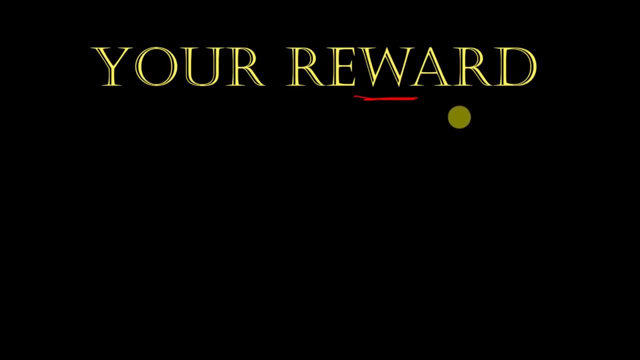 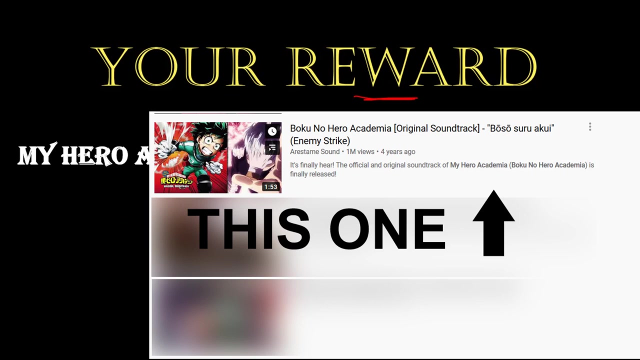 you cool things which i find on internet, like not related to study, things you can enjoy for some time. so in this video, i will share you a song as a reward, which is this one that the my hero academia anime strike named song. the link of this song is in the description box below. this is not at all. 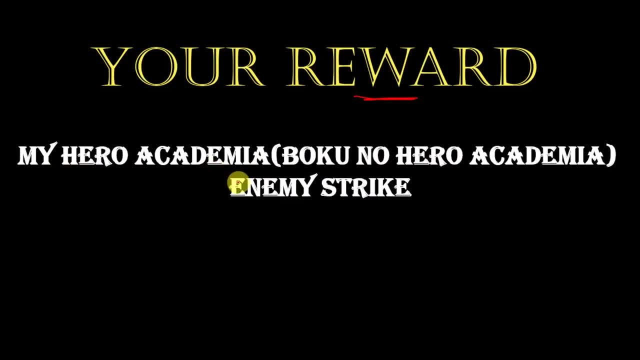 sponsored. nothing like if these guys sponsor me, i will be very rich. so enjoy listening to this song, which is your reward on watching this video. so thanks for watching this video and always remember that math is everything.